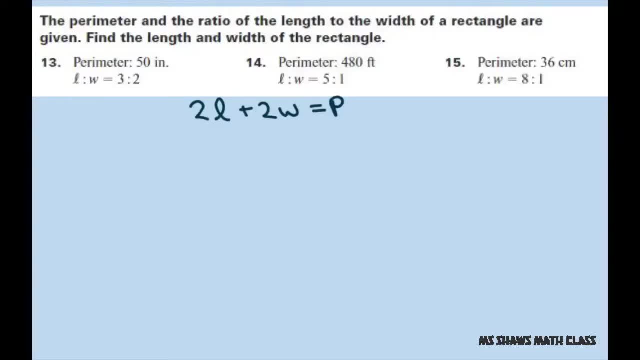 Hi, the perimeter and the ratio of the length to width of a rectangle are given. Find the length and the width of the rectangle And we're going to do these 13 problems. So for 13,, here's our formula. And we know the length to width is 3 to 2.. So we're going to say: 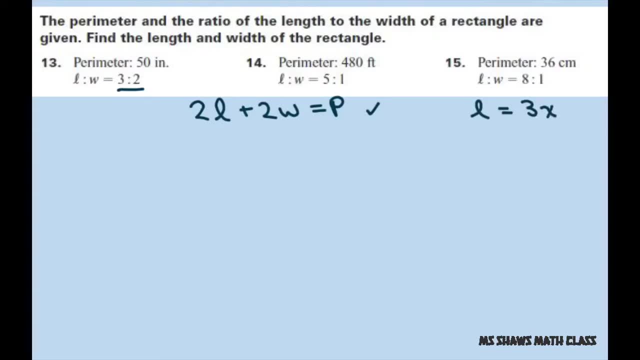 the length is 3x and the width is 2x And fill, use substitution and fill everything in. So we have 2 times 3x plus 2 times 2x equals 50 inches. So you multiply, you get. 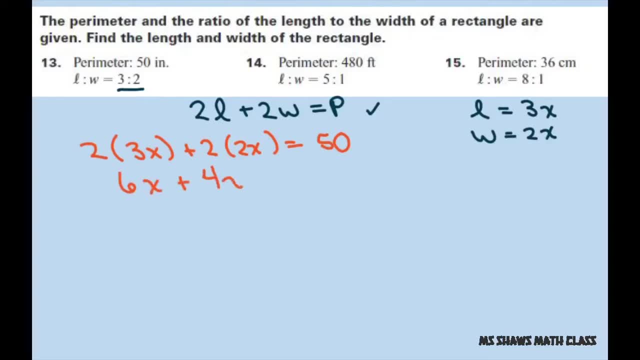 6x plus 4x, 4x equals 50. Combine like terms and divide both sides by 10 and you get x equals 5.. So now you just plug in the length and the width. So basically the length is 3 times 5, which 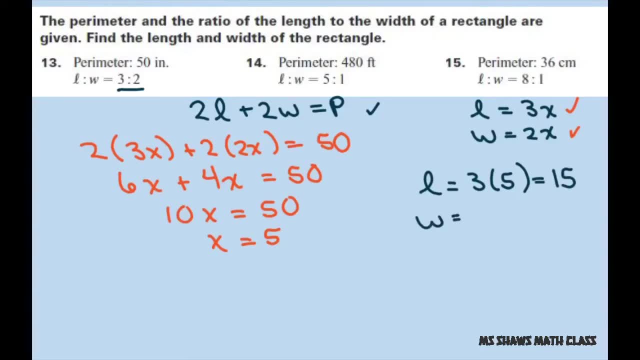 is 15.. And the width is 2 times 5.. And if you wanted to check, you could plug it back in to your formula. So you have 2 times 15 plus 2 times 10 should equal 50. So that would be: 30 plus 20 equals 50, which 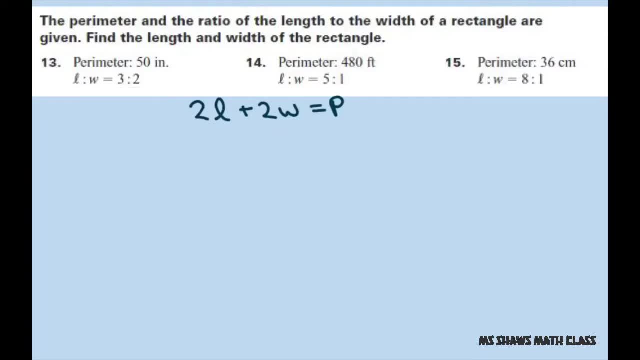 checks out. All right, let's do 14.. So we have: the length is going to be 5x and the width is 1x or just x, So let's fill it in. So we have 2 times 5x plus 2 times x equals 480 feet. All right. 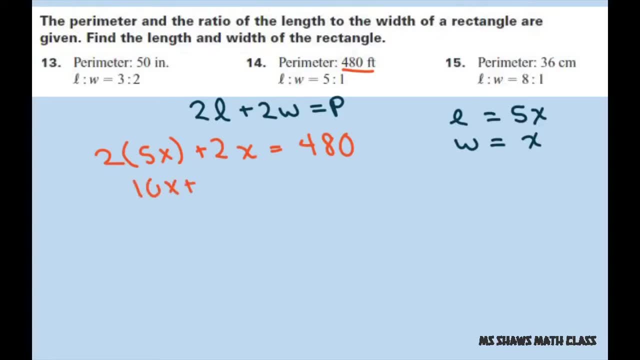 so we have: 10x plus 2x equals 480.. 12x equals 480. And divide both sides by 12. So you get 480 divided by 12.. So you get: x equals 12 goes into 480.. Three times, I believe. 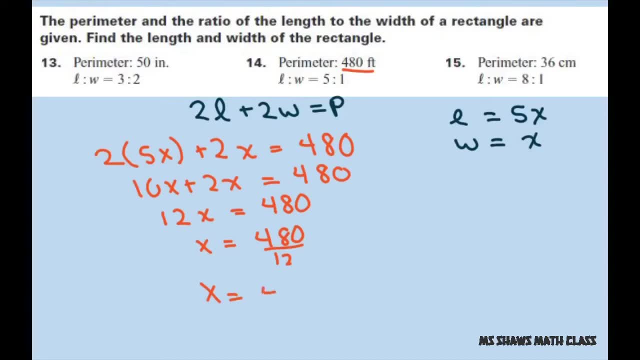 Okay, Four times Four times, And then you still have that zero. So x is 40. Then to find the length and the width, you just do 5 times 40, which gives you 200. And x is just 40.. 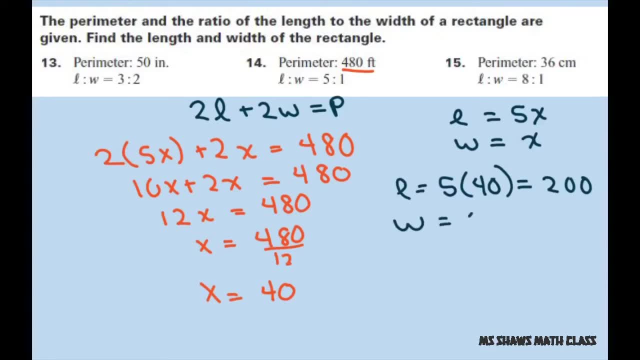 So this is your length, So your width is just 40.. And again, you can plug it in back here to check your answers. All right, And then for the last one we have, the length is going to be 8x and the width is just x. So plug it in: 2 times 8x plus 2 times x equals 36. 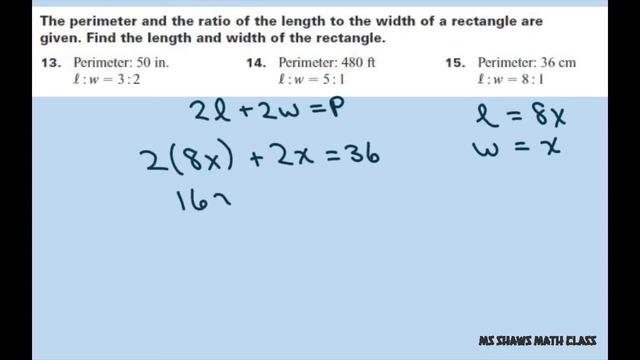 centimeters. So 16x plus 2x equals 36.. All right, All right. 18x equals 36.. Divide both sides by 18.. So x is 2.. To find the length and the width, the length is going to be 8 times 2,, which is 16. And we'll just call it centimeters. 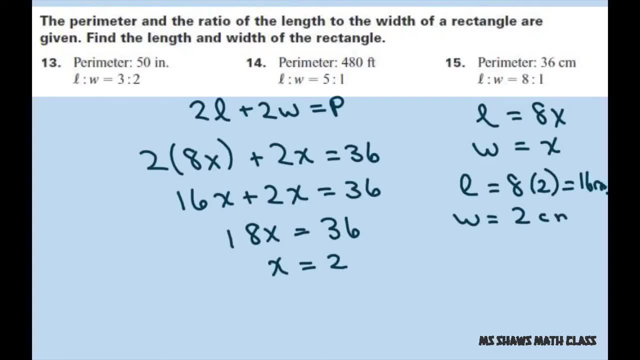 And the width is just going to be 2 centimeters. You want to plug it back in? Let's go ahead and plug this one back in, So we have 2.. All right, 3 times 16.. 7 times 16 centimeters plus 2 times 2 centimeters should equal 36 centimeters. So we have 32. 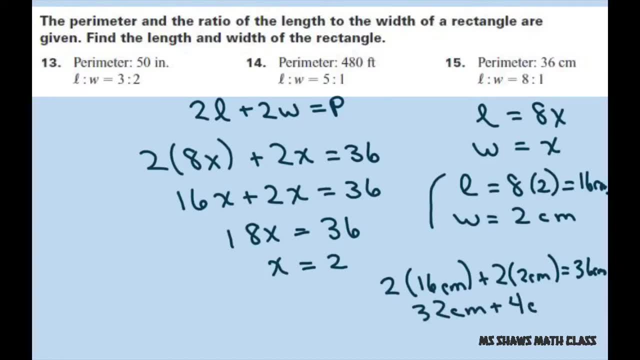 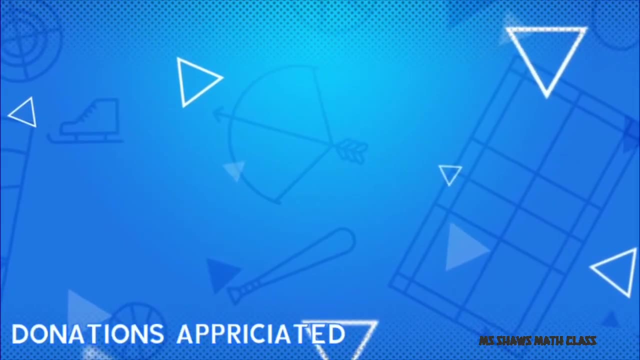 centimeters plus 4 centimeters does equal 36 centimeters, And that's it, Thank you. Have a nice day, Bye-bye. Thank you.